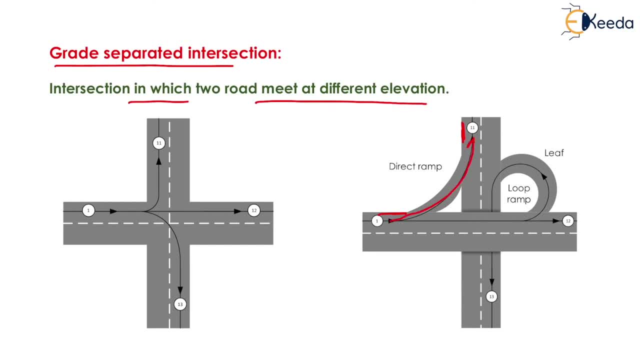 travel from this road to the bottom road, then we have to use the ramp, that is the direct ramp. Now, if we have to merge from this traffic to this traffic that is at the bottom road, then we have to use the loop ramp, just like this. Now the various types of grade separated: 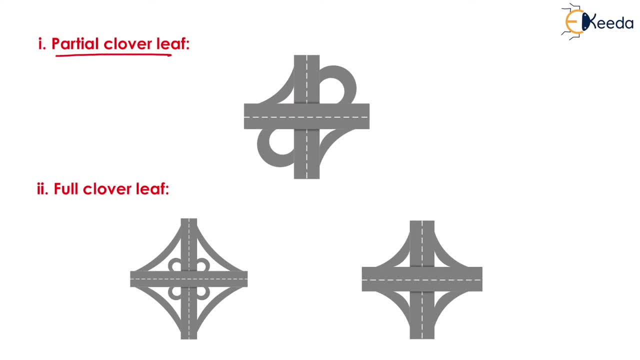 intersections are. the first one is partial cloverleaf, in which cloverleaf is provided partially. that is just like this Now. the next is the full cloverleaf, in which the cloverleaf is provided fully, like this Now, if some vehicle is trying to move from this road to this road. 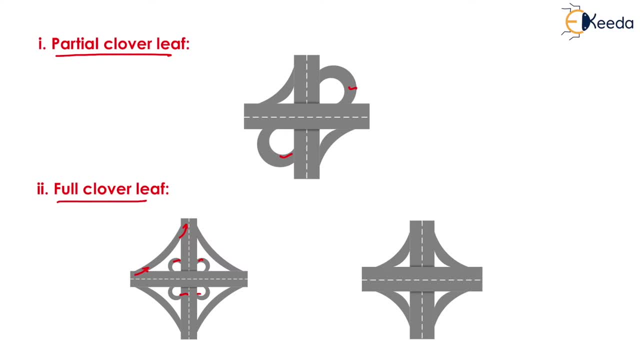 then it will use this ramp. Now, if some vehicle is trying to move from this road to this road, he will use this leaf. Similarly, now, if some vehicle is trying to move from this road to the bottom road, then he will use this leaf, and so on. Now, the next is the at grade intersection, or 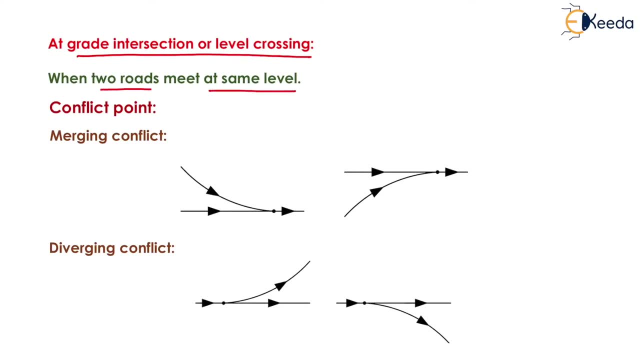 level crossing. When two roads meet at same level, then that intersection is known as at grade intersection. Now there will be conflicts points. Now we will see each type of conflict point, starting with the merging conflict. Now suppose that if one vehicle is trying to move from this road so that he can merge on this road, so there will be one conflict point. 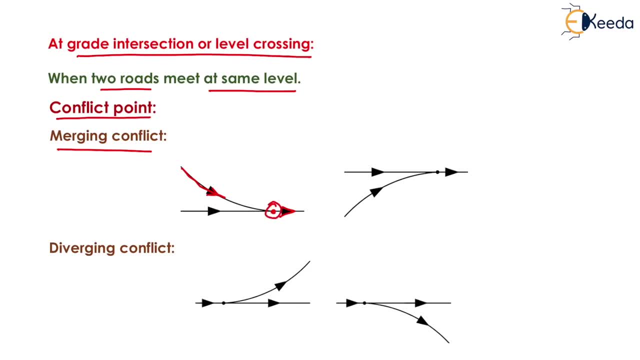 arises here. Similarly, if some vehicle will try to merge from this direction to this direction, then there will be one conflict point, and this conflict point is known as merging conflict. Now, the next one is the diverging conflict, If some vehicle is trying to diverge from this. 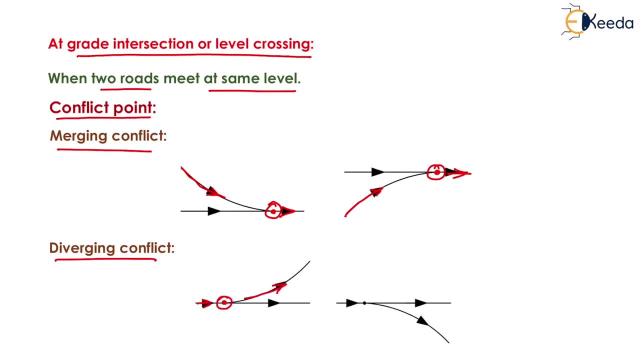 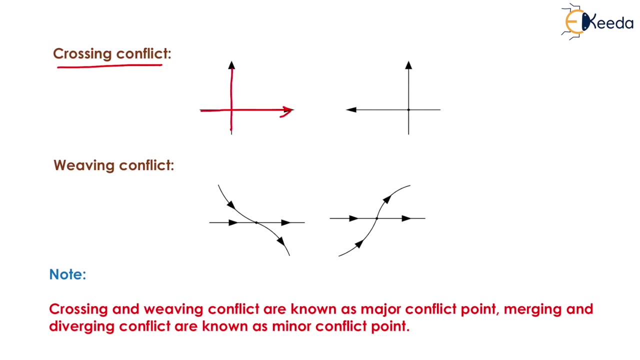 route to this route, then there will be one diverging conflict point that arises here Now. if some vehicle is trying to move from this to this direction, then there will be one diverging conflict point arises here Now. the next is the crossing conflict. Now, if two vehicles are trying to cross each other like this, then there will be one. 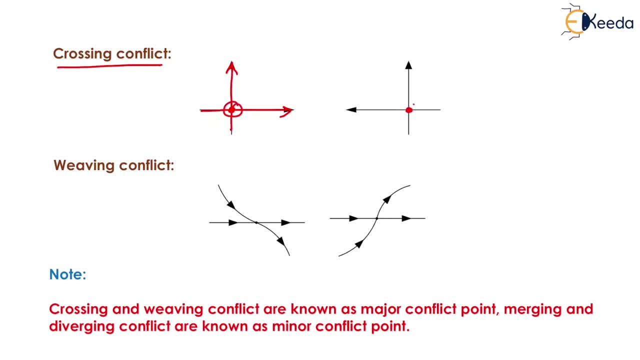 crossing conflict point arises here. Similarly, one crossing point arises here also Now. the next is the weaving conflict. Now, weaving conflict will take place when some vehicle will try to merge from this direction and diverge from this direction. then there will be one. 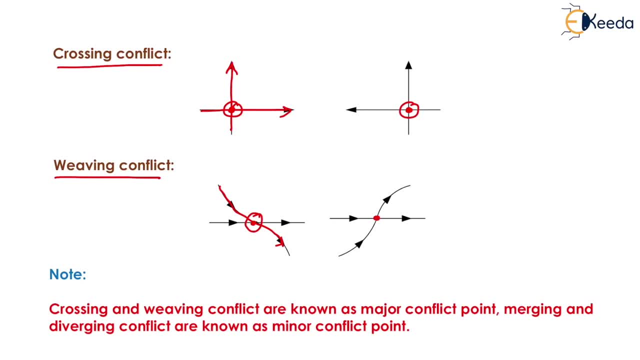 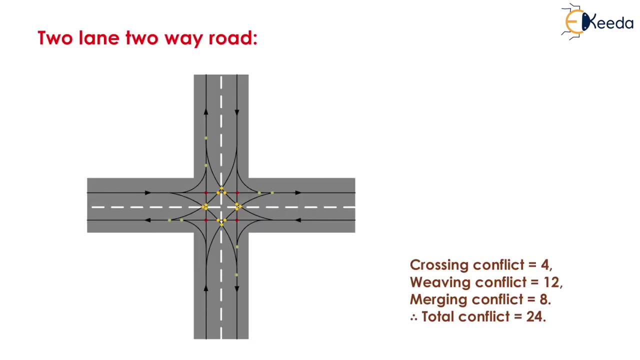 weaving conflict point arises here. Similarly, one weaving conflict point arises here also. Now, one note is written here that crossing and weaving conflicts are known as major conflict point. Merging and diverging conflicts are known as minor conflicts points. Okay, this question is very important from the gate point of view because in 2019,. 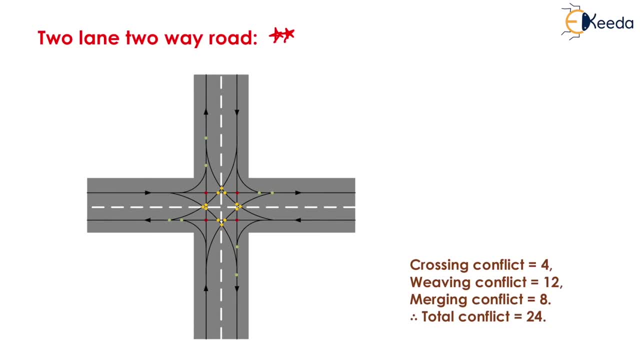 gate had asked the question from this topic. Now we will see the various types of conflicts. point arises in two-lane, two-way road. Now this vehicle will move just like this and it will take the path just like this, or it will take the path. 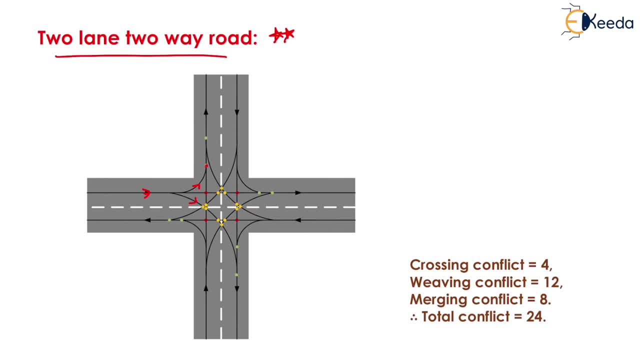 just like this. So there will be one merging conflict as well, as there will be one merging conflicts also there. that is at this point Now. similarly, if this vehicle is trying to change its path from this direction to this direction or from this direction to this, 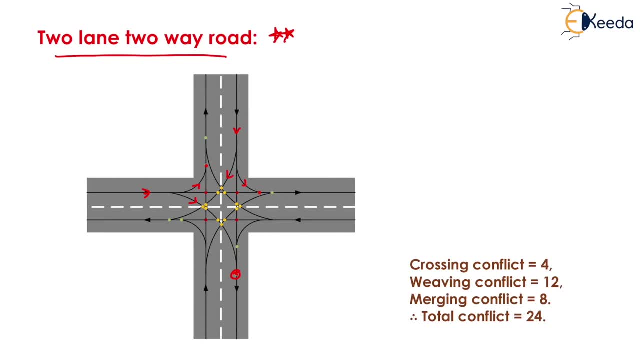 direction. then there will be one merging conflicts or there will be one merging conflict. Similarly, there will be also one merging conflict as well, as there will be one merging conflict. similarly, there will be one merging conflicts and there will be one merging conflict, so total. 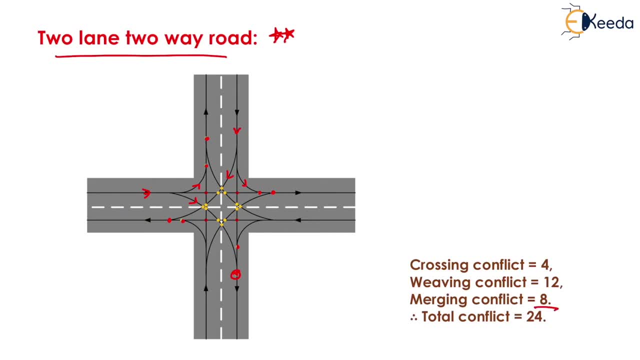 merging conflict will be equals to 8. here now, crossing conflict will be just like this. that is the crossing conflict as well, as this is also crossing conflict, this is also crossing conflict and this is also crossing conflicts. so crossing conflict will be equals to 4 and weaving conflict. 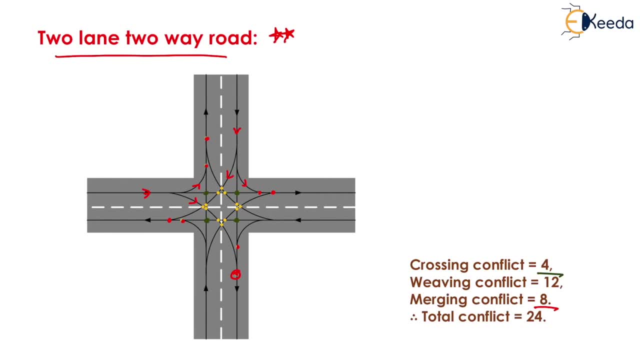 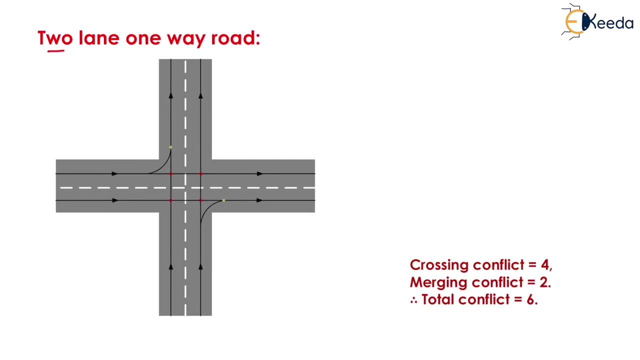 will be shown here by the yellow color. these all are the weaving conflicts, so it will be equals to 12. so on adding these three conflicts, the total conflict will be equals to 24. so for two lane two-way road, the total conflict point will be equals to 24. now for two lane one-way road, the 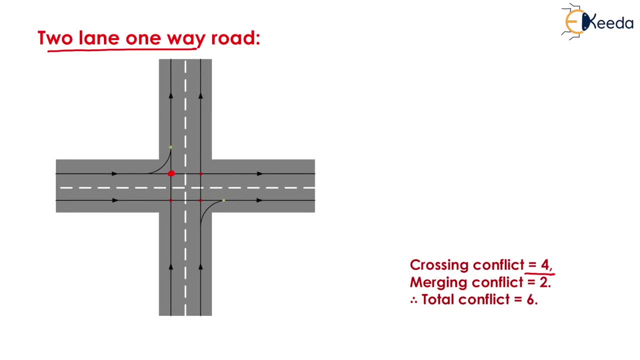 crossing conflict will be equals to 4, which is shown here. that is this, and merging conflict will be equals to 2, which is shown by green dots. so total conflict will be equals to 6 in two lane one-way road. now we have the conflict points of different types of road. 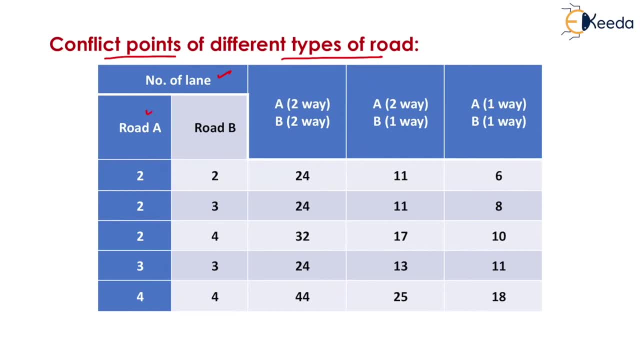 in the first column we have written number of lane for road a and for road b, if road a has two lane as well as road b also has two lane. now if road a is two-way road and if road b is two-way road, then there will be 24 conflicts points. similarly, if road a is two-way and road b is one way, 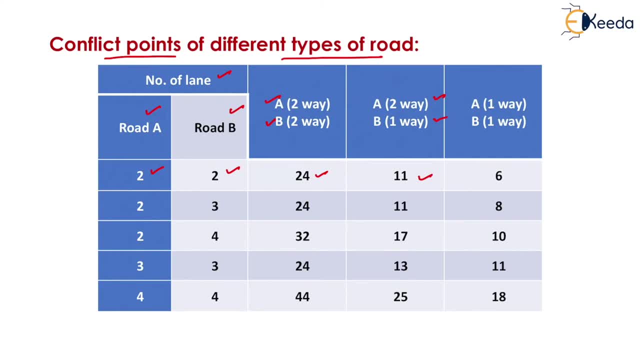 then there will be only 11 conflict points. now. if road a is one way and road b is one way, then there will be only six conflicts points. now. these conflict points are important from the gate point of view because gatehead are several time these conflict points. 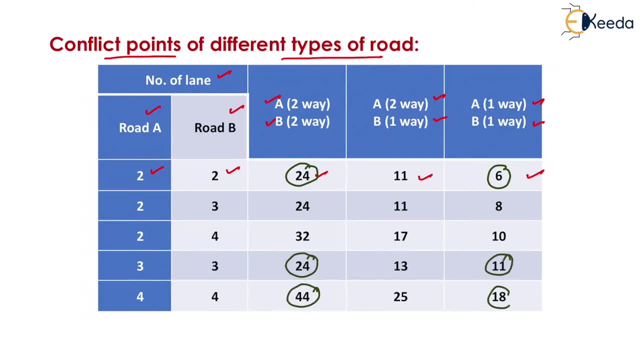 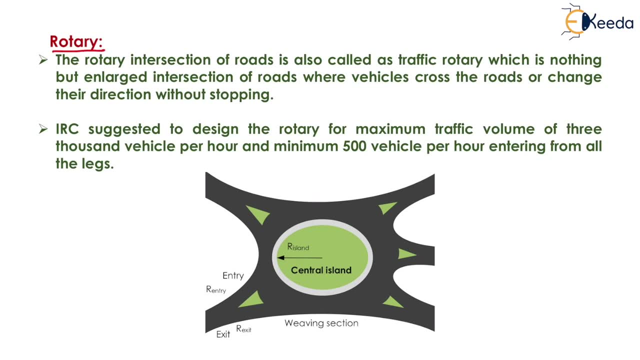 so we will encircle these conflict points. okay. now, in the similar way, we can determine the conflict point for all the other cases also. now the next topic is the road tree. the road tree intersection of road is also called as traffic road tree, which is nothing but a light intersection of road. 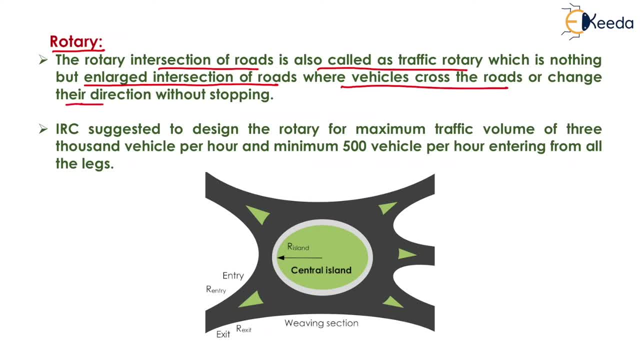 where vehicle cross the roads or change their direction without stopping. irc suggested to design the road tree for maximum traffic volume of 3000 vehicle. now, this is very important. this condition is very important. that is, the maximum traffic volume suggested for the design of rotary is 3000 vehicle per hour and 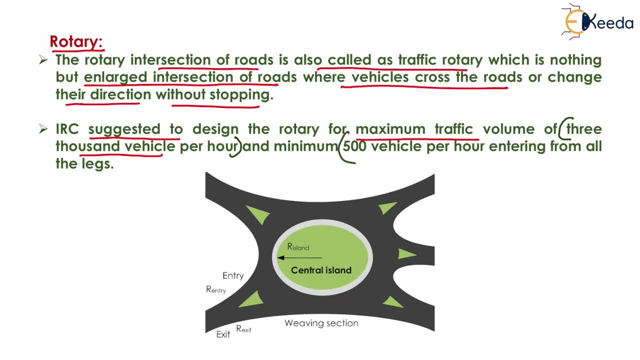 the minimum number of vehicle is 500 vehicle per hour. this is very important from the government exam point of view, entering from all the legs. now here a rotary shown just like this, and here is different roads, just like this. that is, the different roads connecting at the rotary. now 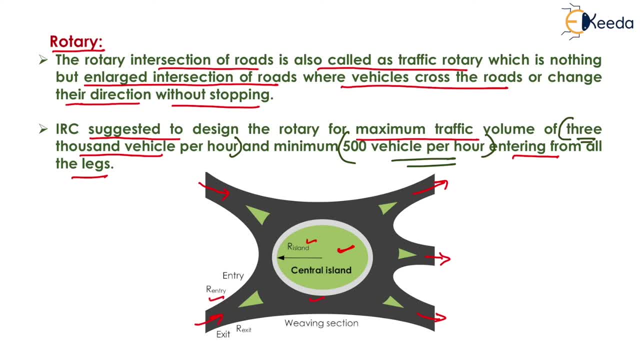 this is the radius of the island, this is the radius at entry and it is the radius at exit. similarly, these are the islands which are provided just to reduce the chances of accidents. now we have the various types of rotary. the first one is circular rotary, which is shown here, in which 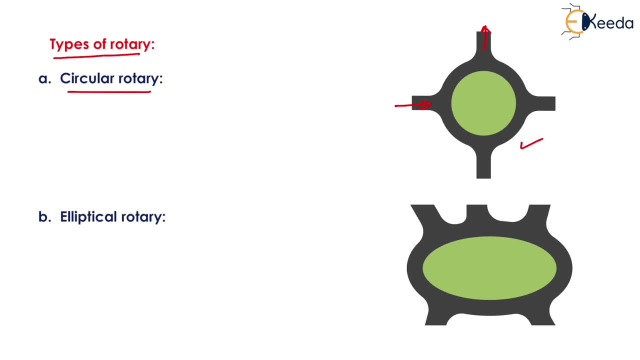 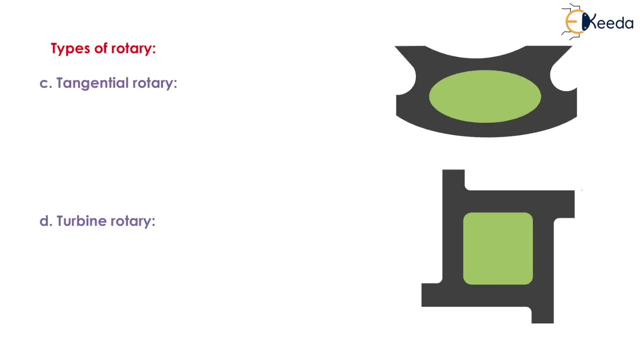 one path will be just like this, one path will be just like this, another path will be just like this and another path will be just like this. good, and here is the central island. Similarly, the elliptical rotary will be just like this, the tangential rotary will be just like this and the turbine rotary will be just like this. 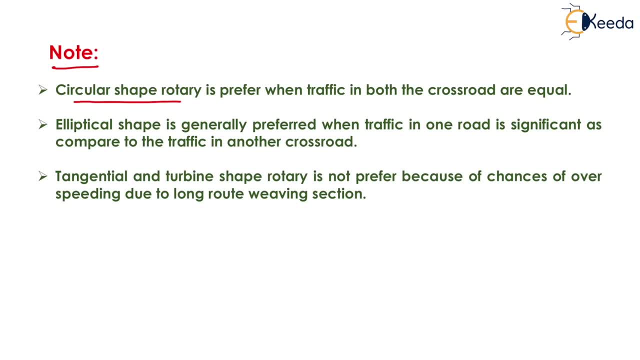 Now, note is written here that circular shaped rotary is preferred when traffic in both the crossroads are equal. Similarly, elliptical shape is generally preferred when traffic in one road is significant as compared to the traffic in another crossroad And tangential and turbine. 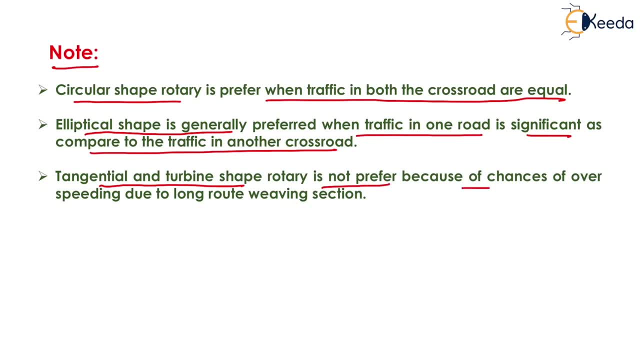 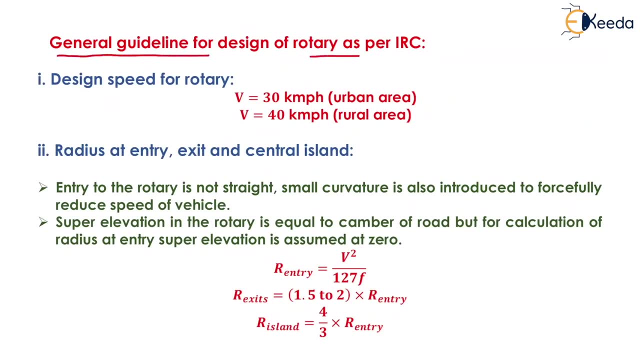 shape rotary is not preferred because of chances of over speeding due to long route weaving section. Now the general guideline for design of rotary, as per Indian Road Congress, Design speed for rotary will be equals to 30 km per hour for urban area and 40 km per hour for rural area. 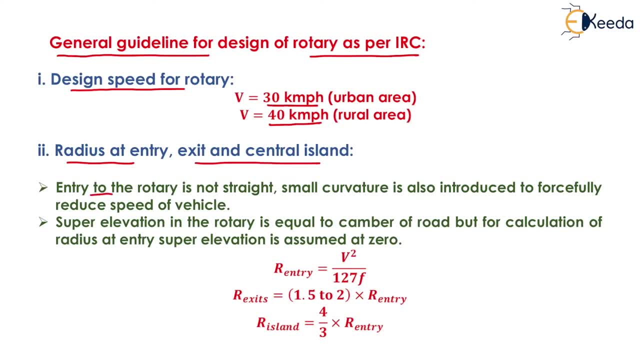 Now radius at entry, exit and central island Entry to a rotary is not straight. small curvature is also introduced to forcefully reduce speed. Speed of vehicle super elevation in the road tree is equals to camber of road. But for calculation of radius at entry super elevation is assumed at zero. So radius at entry will be equals to V. 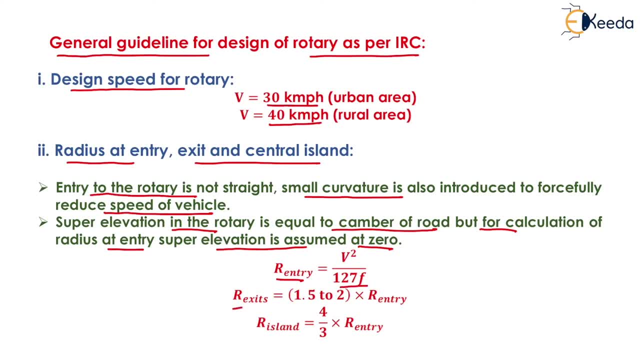 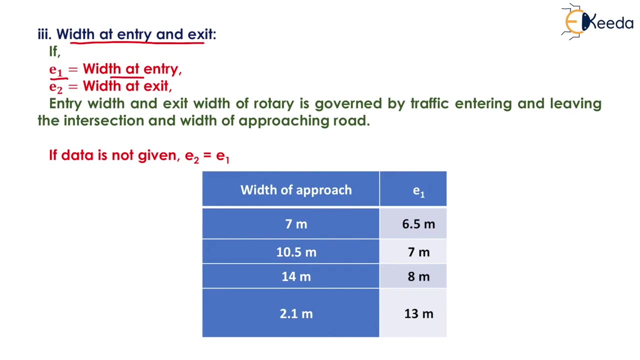 square upon 127 F, and radius at exit will be equals to 1.52 times of radius at entry, as well as radius of island will be equals to 4 by 3 of radius at entry. Now, width at entry and exit: E1 is the width at entry and E2 is the width at exit. Entry width and exit width of road tree. 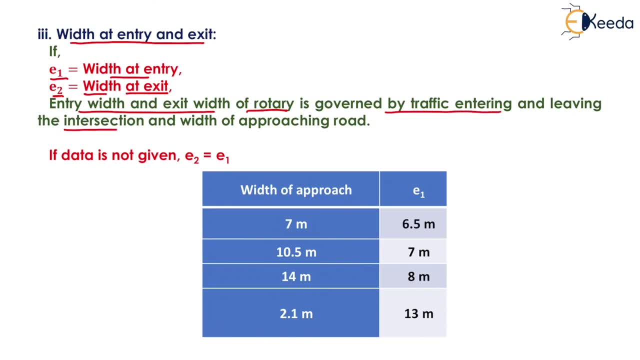 is governed by traffic entering and leaving the intersection and width of the approaching road. Now, if data is not given, than we have to take. the width at exit will be equals to width at entry. Now we have the width at approach, that is the road width, and we have 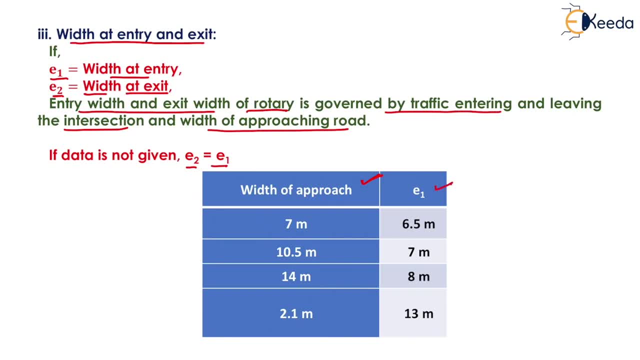 the width at entry, that is even now. for 7 meter width of approach even will be equals to 6.5. similarly, for 10.5, even will be equals to 7 meter. for 14 meter, approach even will be equals to 8 meter. and for 21 meter approach even will be equals to 13 meter. now, length of weaving section. 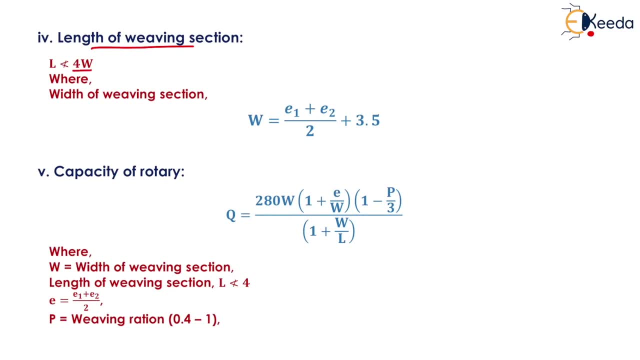 will not be less than 4 times of width of weaving section. now w will be equals to even plus e2 by 2 plus 3.5. now the next is the capacity of road tree: it will be equals to 280 into w 1 plus e by 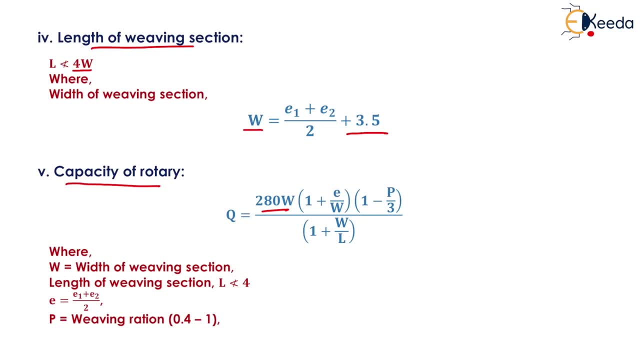 w, 1 minus p by 3 upon 1 plus w by l, where w is the width of weaving section, l is the length of weaving section, which should not be less than 4 times of width of weaving section. e will be equals to even plus e2 by 2 and p is the weaving ratio generalized in between 0.4 to 1. that is all about.